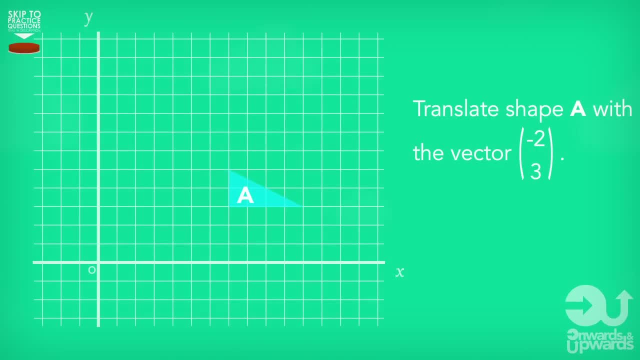 So if we have shape A, we might be asked to draw where shape A would be if we translate it with the vector minus two, three. So one good, quick way of doing these questions is to pick a single point on our shape like this, and we're going to use this as our starting. 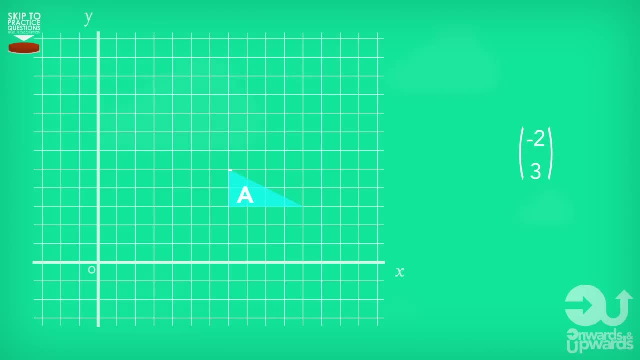 point. First we look at the top number to see how far- left or right- the shape needs to move. Then we look at the bottom number to see how far up or down the shape needs to move. So in this case we move two across to the left and then we move three up and 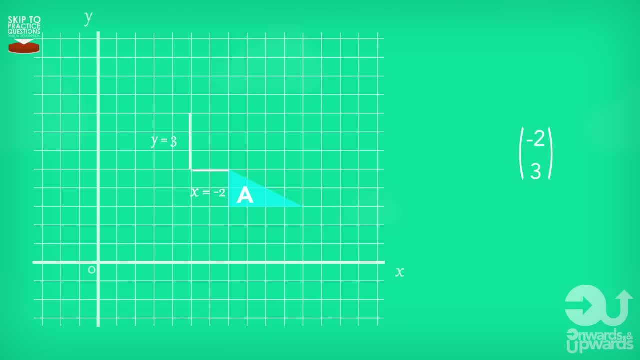 that's where we move our starting point to. Now. we can just draw our original shape around this point. So we know from the first point that we draw a straight line down roughly about that long, and another line across roughly about this long, and the last line can just: 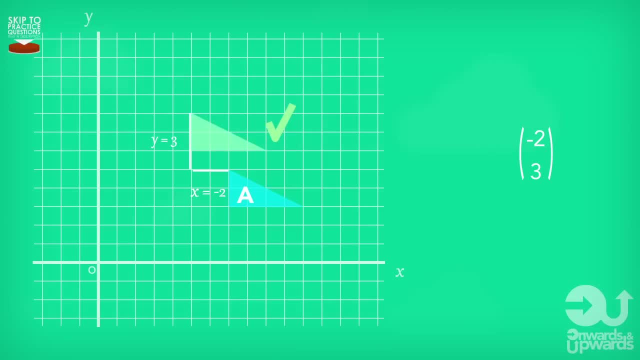 join the two points together. However, if you're using this method, be sure that when you draw the final shape, it's the same as the original shape in every way- Another, slightly longer but more reliable way of doing these questions that also avoids any risk of drawing the shape incorrectly. 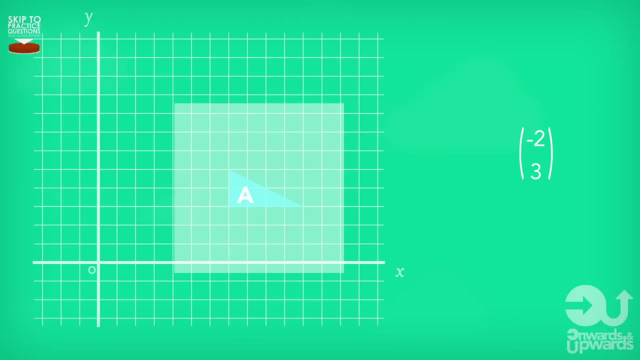 when we do the final shape is basically just to use tracing paper. Using this method, we draw the whole original shape, Then we move our starting point, exactly like we did before, according to the column vectors, but this time we move the whole tracing paper. Now we can see exactly what the shape will. 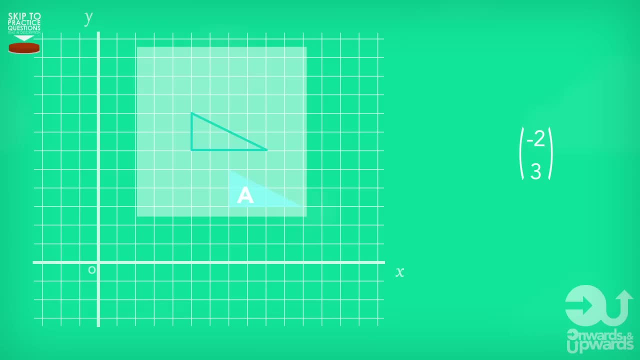 look like and where the shape will be when we've moved it. And once you've done this, you can just draw in the actual shape on the sheet of paper. And once you've done that, it's game over. job done collection medal you've won. 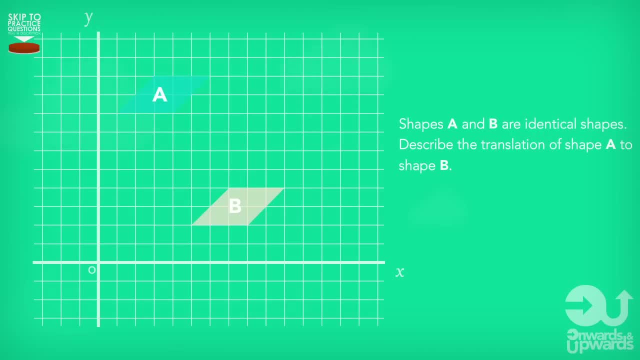 So here's another type of question. Shapes A and B are identical shapes. Describe the translation of shape A onto shape B. Now, with these questions, all we do here is pick a single point of the shape- once again our famous starting point. Then we need to track down how far away the point is on the